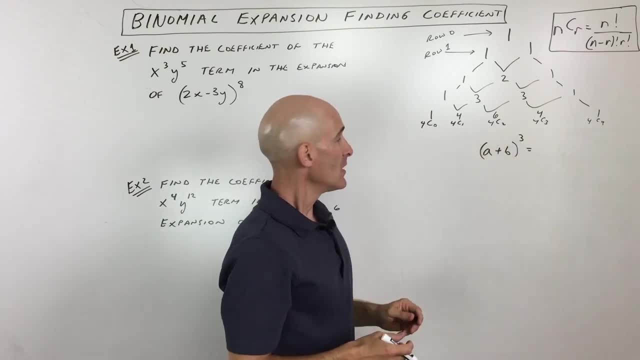 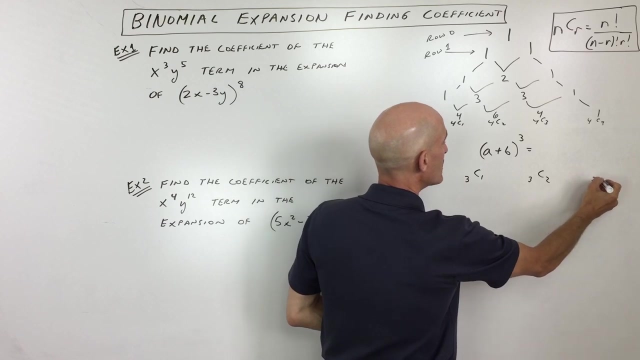 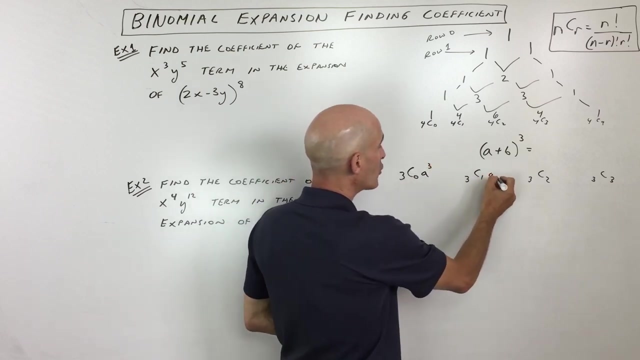 So, for example, say we wanted to expand a plus b to the third power. What we can do is we could say: well, let's go down here to the third row, and these are our coefficients: one, three, three, one. The other way to do it is to go like this: we could say: three choose zero. three choose one. three choose two, three choose three. Then what you do is you take the first term- okay here, a- and you go to the third power and you go in descending order: a squared, a to the first, a to the zero. Then you take the second term, b. 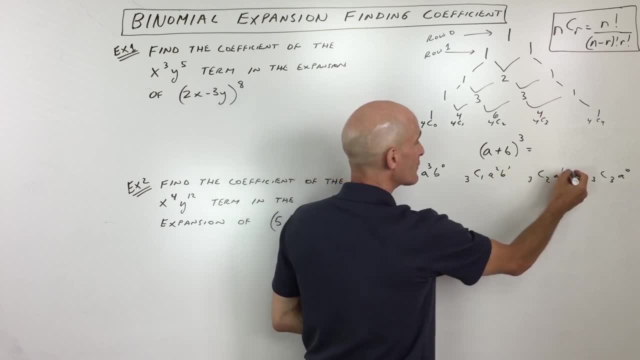 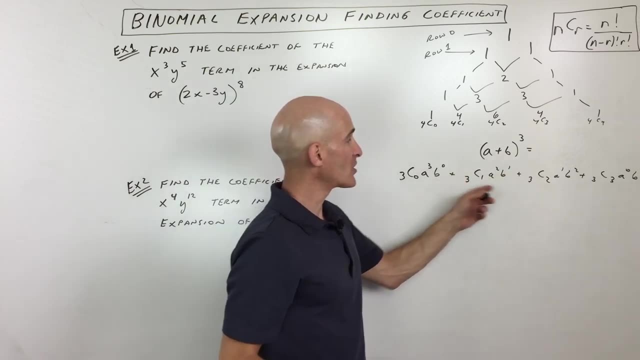 and you go in ascending order, so b to the zero, b to the first, b to the second and b to the third, And then these terms are all added together and you can go ahead and simplify and those are going to be the terms in the expansion of a plus b to the third power. Now I want you to notice a pattern here that will be very helpful. See how we're on the third power. we're also on the third row here. see this: three choose zero. Notice how the second term. see the b- b to the zero power, and see how this is: three choose zero. 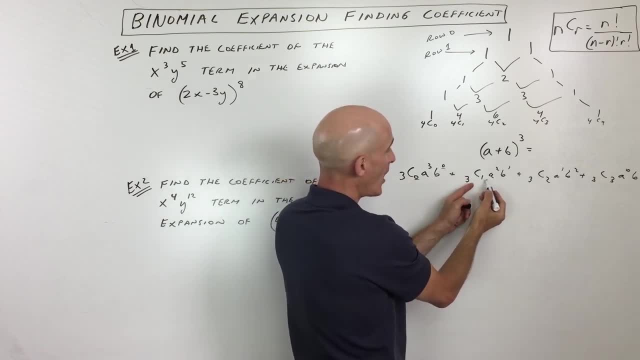 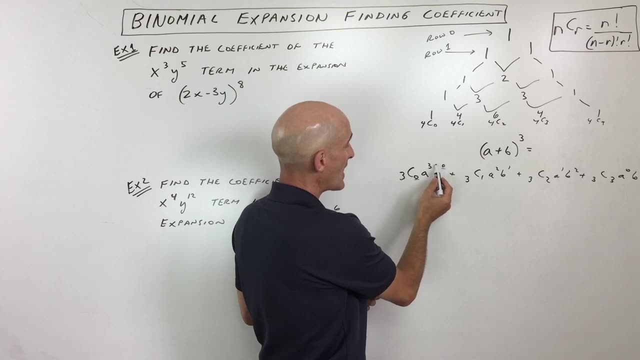 See how these guys match Same thing over here: See 3, choose 1.. B to the first power: See 1 and 1.. The other thing I want you to notice too, is that see how 3 plus 0 adds up to 3.. That's the power. 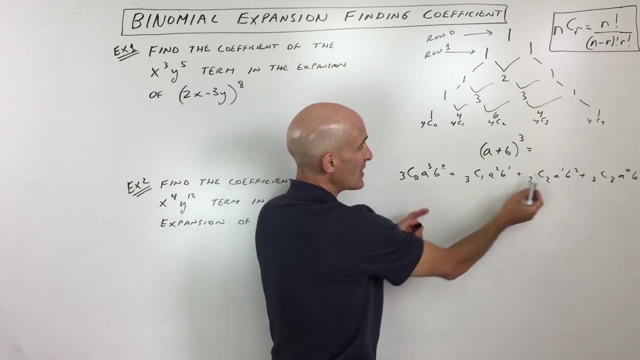 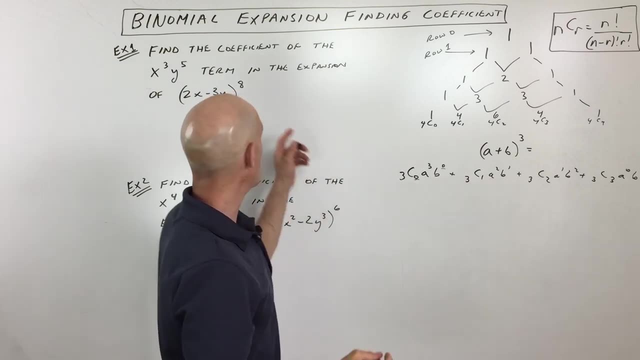 here. That's also the row. okay, 2 plus 1 is 3.. 1 plus 2 is 3.. So if you recognize that pattern, you can use that to find a specific term in this expansion. So I'll show you over here. 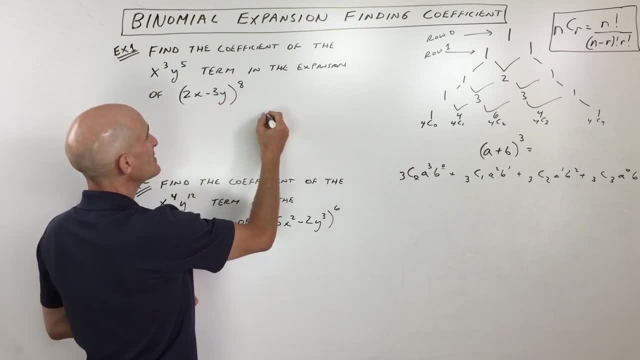 So, for example, 2x minus 3y to the 8. We can see that our two terms are 2x and negative 3y. Now I'm capturing this minus as a negative 3y, And then we want this to be x cubed. So I'm going to make 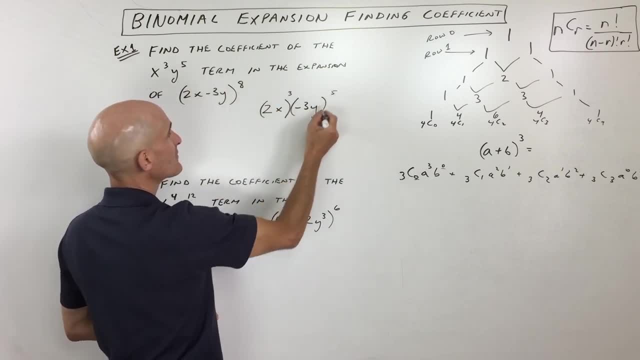 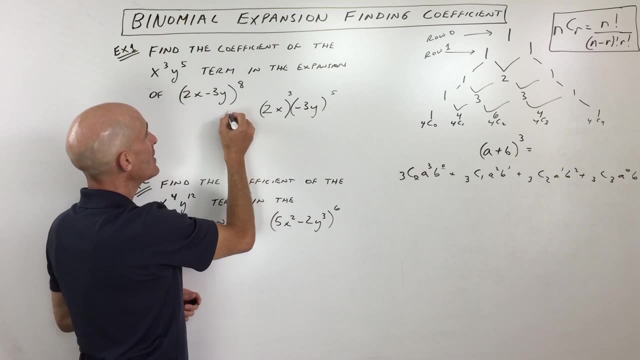 this to the third power. I'm going to make this to the fifth power to give us y to the fifth. Now notice, we're on the eighth power. So that's the eighth row. If we were to expand this down Pascal's triangle, this is going to be 8, choose. What do you think goes here? Well, 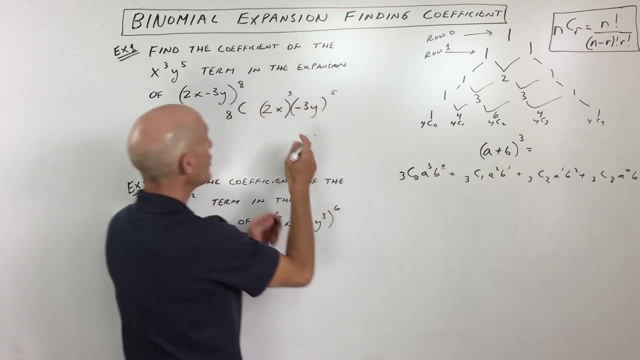 remember the pattern: See 0,, 0,, 1,, 1.. 2,, 2, and so on. So if this is 5, this is going to be 5 as well. So now all we have to do is we're. 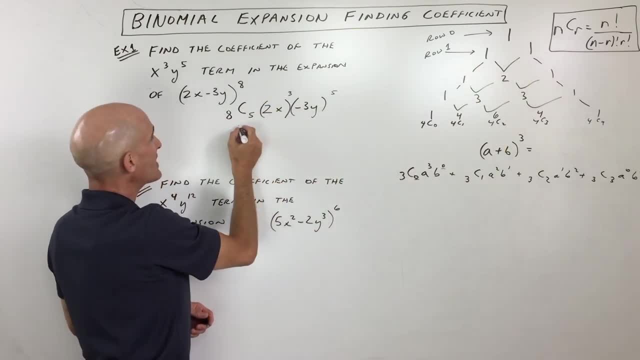 going to use the formula over here for combinations. okay, So 8, choose 5.. That's 8 factorial over 8 minus 5, 3 factorial times 5 factorial, And then we've got 2x cubed, which is 2 cubed is 8,. 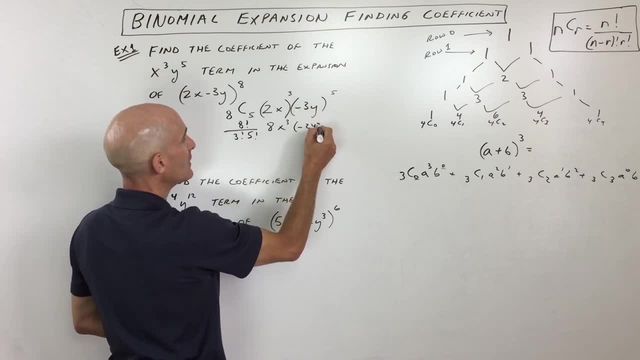 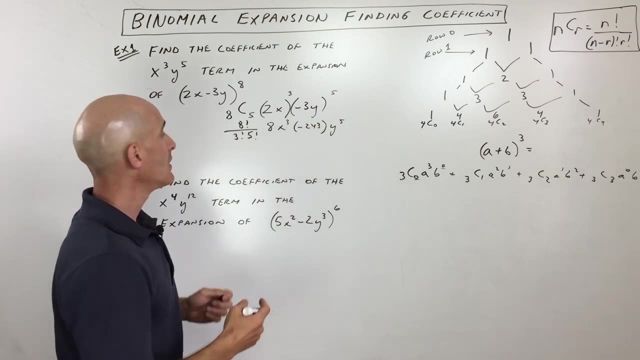 okay, Negative. 3 to the fifth is negative 243y to the fifth. Now, all we have to do now is simplify all the numbers. That's going to be our coefficient in front of the equation x cubed y to the fifth term. So 8 factorial is really like 8 times 7 times 6 times 5, all the way. 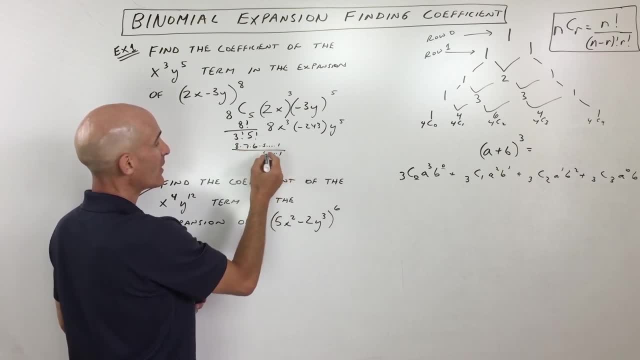 down to 1.. 5. factorial is 5,, 4,, 3, 2 multiplying all the way down to 1.. So you can see those are canceling. 3, factorial is 3 times 2 times 1, which is 6.. So you can see those are canceling. So now, 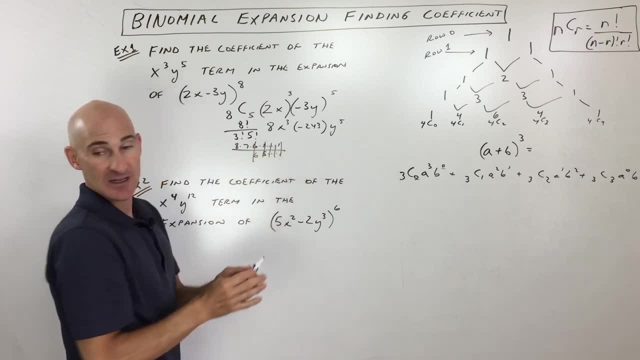 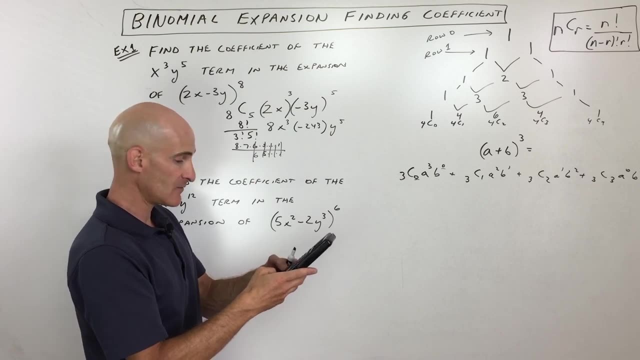 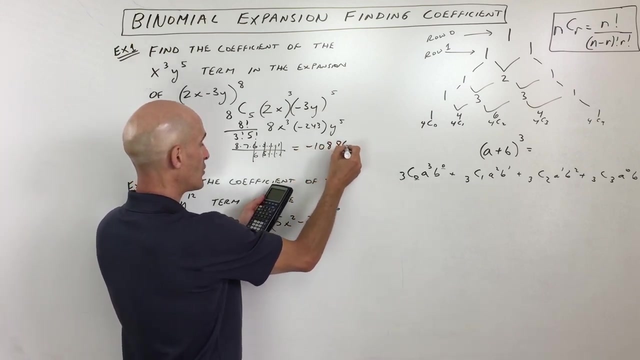 we can see we have 8 times 7, which is 56 times 8 times negative 243. So let's go to the calculator here. We've got 56 times 8 times negative 243. So that comes out to negative 108,000, negative 108,864, x cubed y to the fifth. Now, if they just 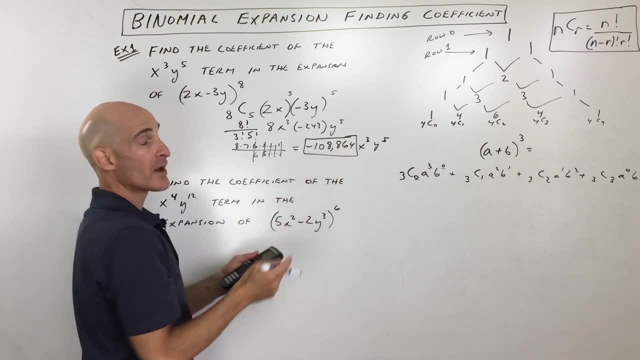 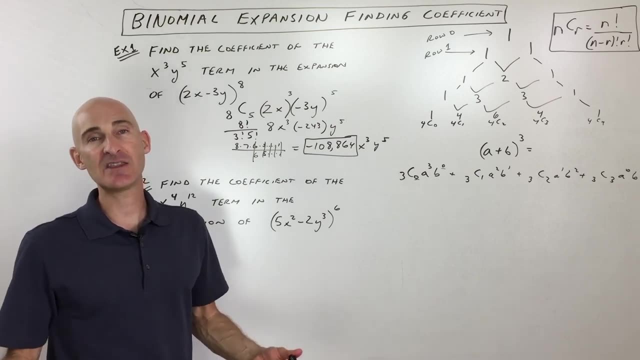 want that coefficient, you would just write down the negative 108,864.. So we're going to do another example. but I know a lot of students right now are preparing for the ACT and the SAT, especially the math section. So I just wanted to let you know about my two math review courses. I've got a huge 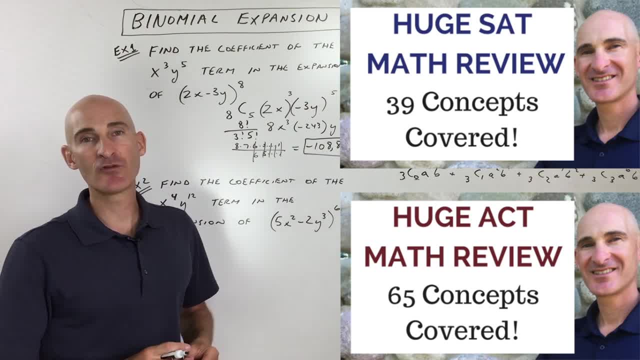 ACT math review video course and a huge SAT math review video course. So check out those video courses. There's three free lessons in each of those courses, So if you take those, you'll get a lot of benefit just from going through those lessons And then you'll get an idea about what the other lessons are going to. 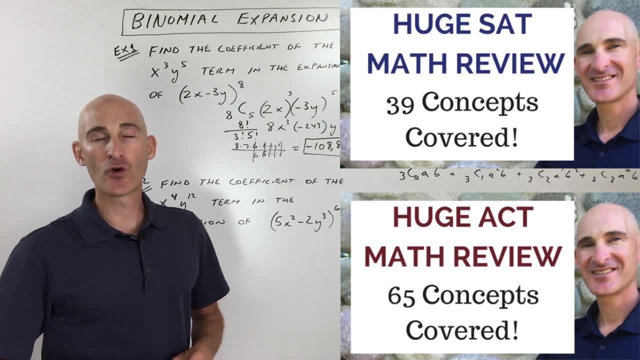 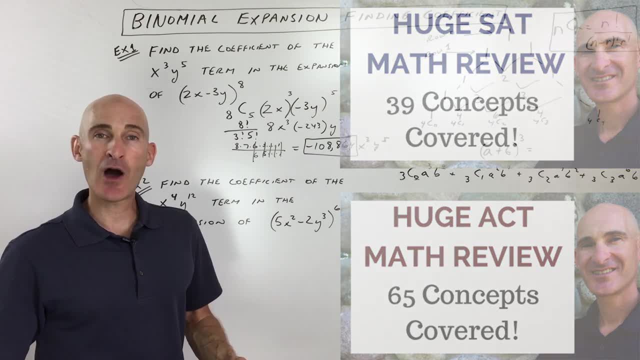 be like as well, And if you're interested, you can go on and purchase that and go through the rest of those. A lot of students have reported back that they've been able to boost their scores utilizing those courses that I put together, So check them out. Otherwise, let's go to example. 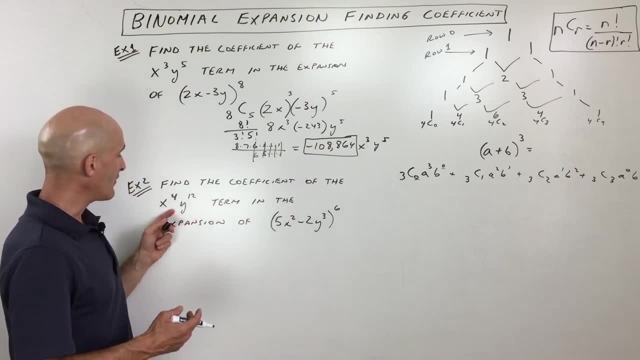 number two. It says: find the coefficient of the x to the fourth, y to the 12th term in this expansion. Okay, so we're already a little bit more experienced now. So we say hmm, x to the fourth, y to the 12th. Well, you can see, these are our two terms, right here, right in our binomial. 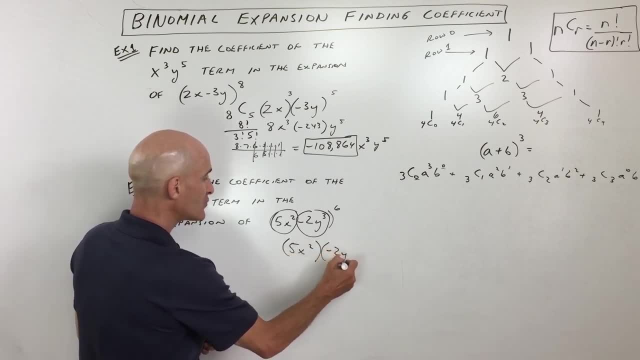 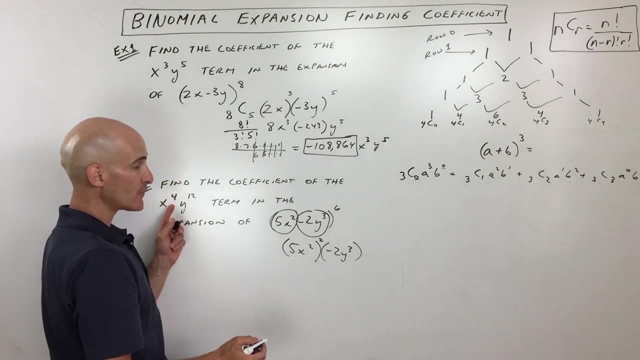 Bi means two right, So 5x squared, and negative, 2y to the third. I want this to be x to the fourth. That means this has to be two, because a power, to power you multiply, that's going to give us the x. 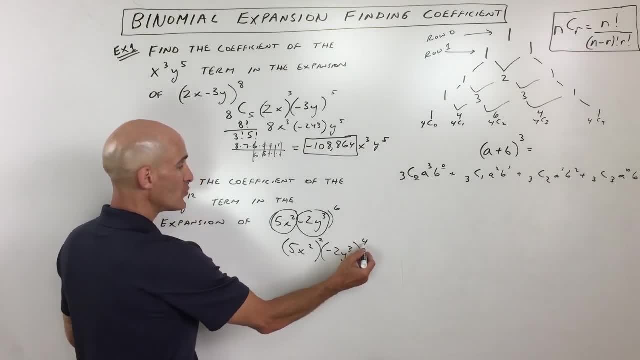 to the fourth. This I want to be four, because yq To the fourth power, three times four gives us 12.. We're on the sixth row, sixth power. So this is going to be six. choose And remember the pattern. See how this is: three. choose, zero. b to the zero. 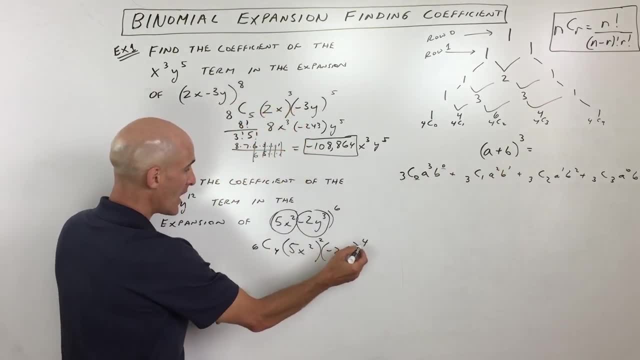 three choose one. b to the one. This is going to be six choose four. See how these match. Now, all we have to do is simplify this out, And that's going to be the particular term that we're looking for, So let's do that. So six choose four. If we use our binomial- I'm sorry, our. 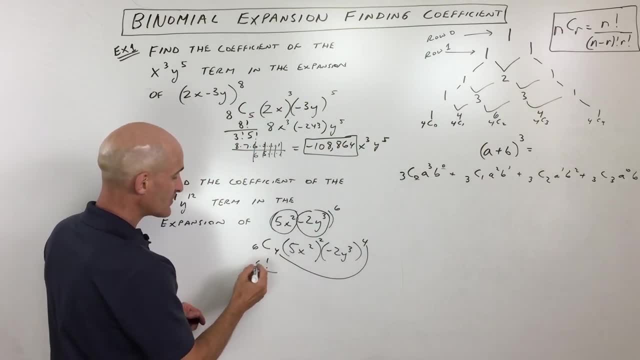 combination formula. right up there we've got six factorial over six minus four. two factorial Times four. factorial Five squared is 25x to the fourth. Negative two to the fourth is 16y to the twelfth, And let's simplify this. So six factorial is six times five times four, all the way down to. 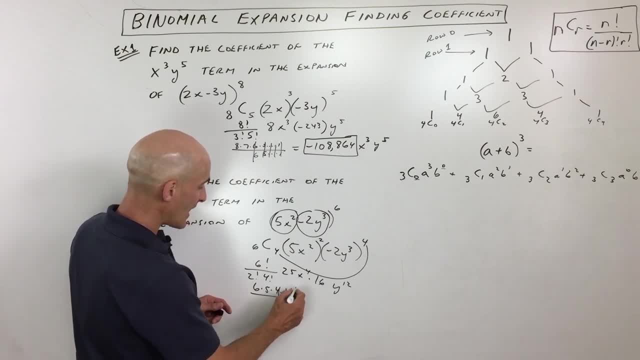 one. Four factorial is four all the way down to one, So those are canceling. And then two, factorial is just two times one. So this is 30 over two, which is 15 times 25 times 16x to the fourth, y to the twelfth. Now we're only interested in the coefficient, So we just have to multiply. 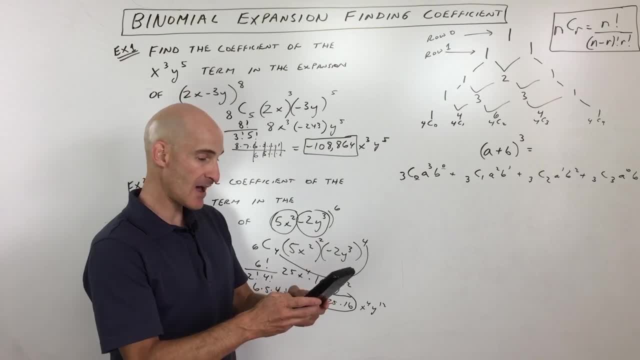 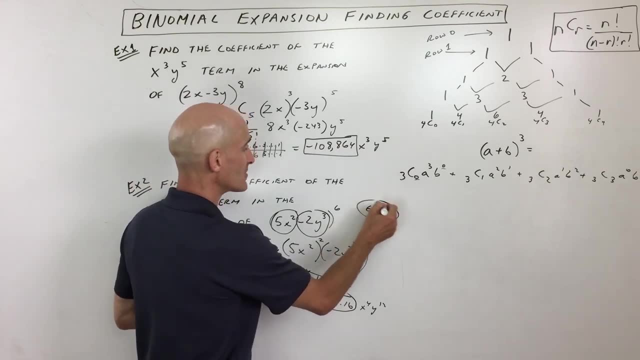 those values out right there. So that's going to be 15 times 25 times 16.. Let's see that's 6,000.. So our coefficient in this particular example is going to be 6,000.. So I hope that helped you how. 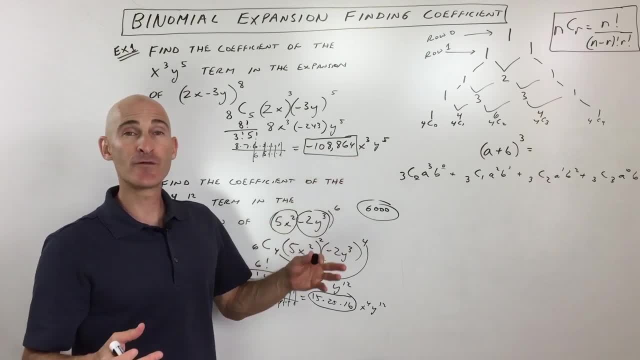 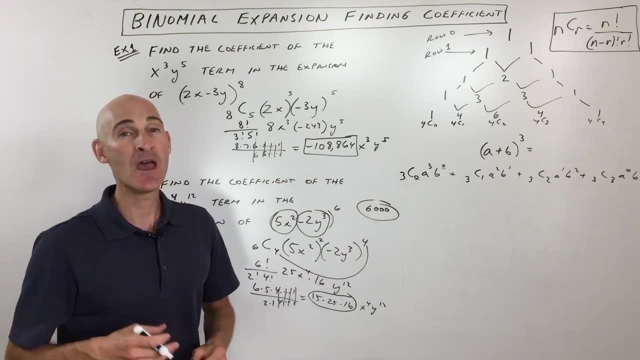 to understand working with binomial expansion theorem a little bit better. I have another video that I can link to if you want to do more problems with binomial expansion, But this is specifically focused on finding the coefficient, So I hope that helps you understand a lot better. 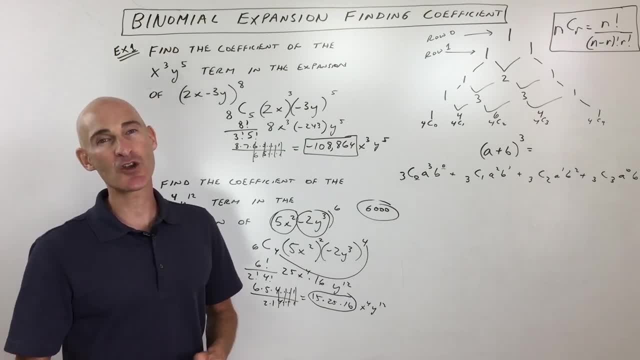 Subscribe to my channel And I'll see you in the next video. Subscribe to the channel. Check out more math videos on my YouTube channel, Mario's Math Tutoring, And I look forward to helping you in the future math videos. I'll talk to you soon.